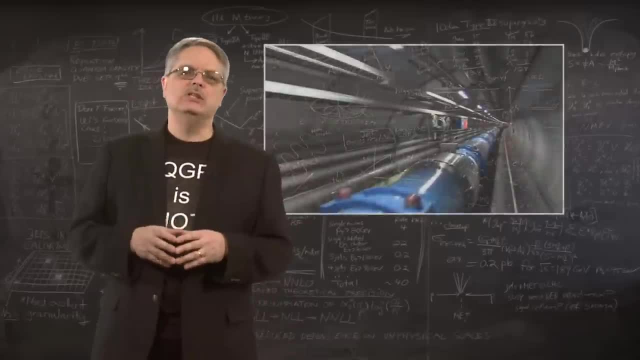 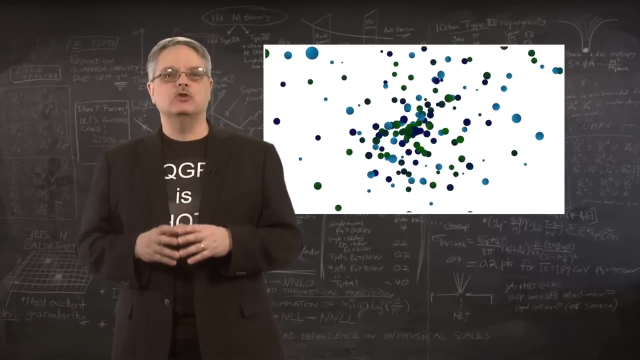 and me to study the laws of nature. Using huge particle accelerators, we can smash beams of subatomic particles together at near the speed of light and generate temperatures a million times hotter than the center of the sun. We particle physicists do have the coolest toys. 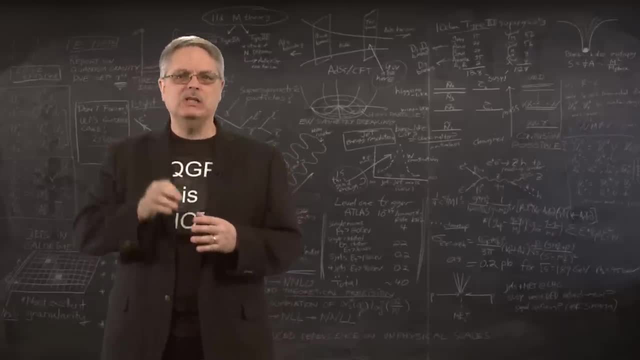 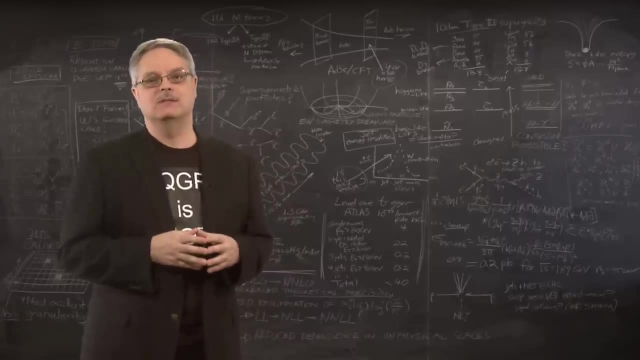 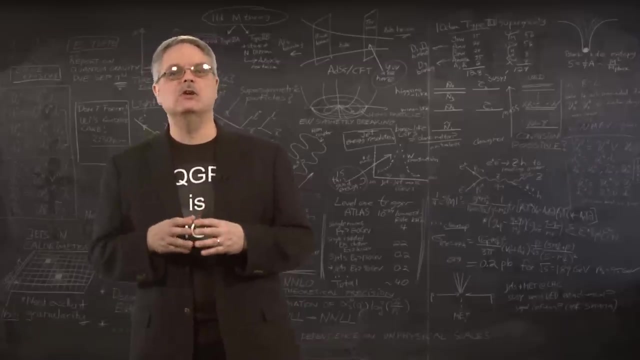 Well, hottest, but you know what I mean. A really interesting thing to think about is what happens to ordinary matter when it encounters temperatures like these. To understand that we can remember some familiar phenomena and then learn about some more exotic things that you might not have heard about before. 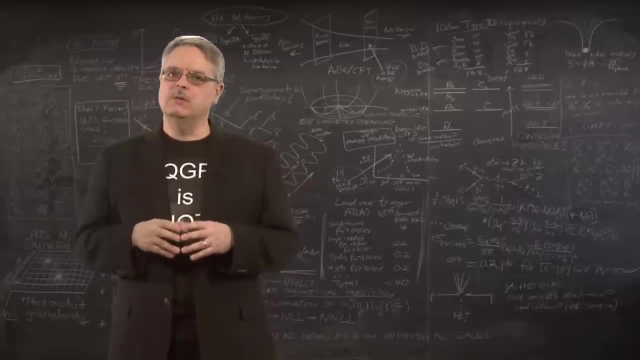 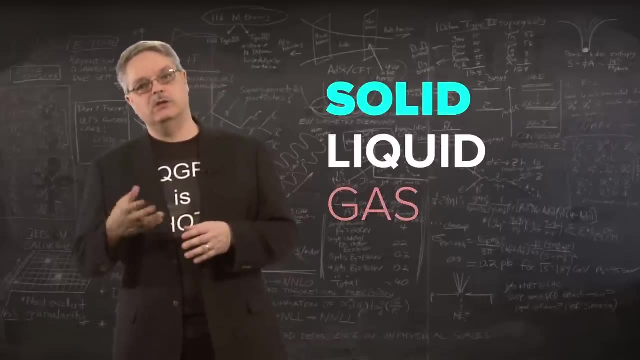 To begin with, we know about the states of matter that we learned about in school, specifically solid, liquid and gas. Of course, things are solid when they're cold, gaseous when they're hot, and they're hot and liquid when they're in between. 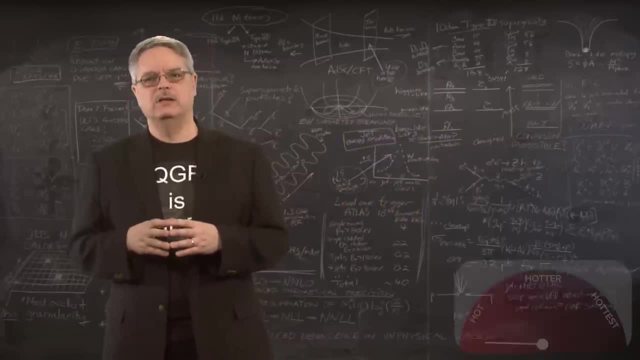 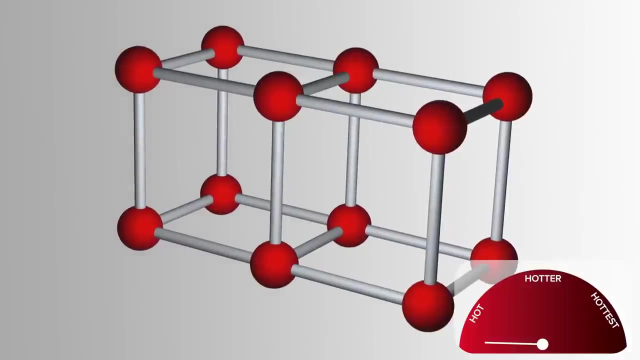 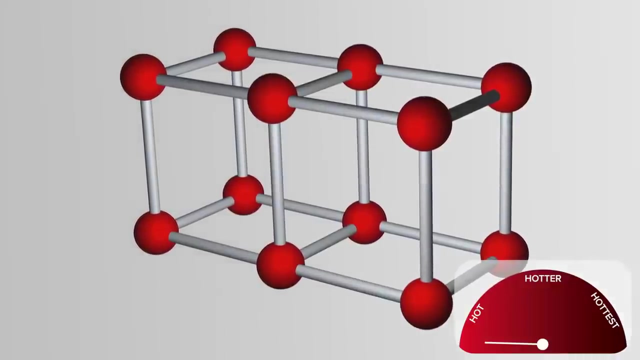 So how does temperature affect the structure of matter? To understand that we need to think both molecularly and atomically. In solids, molecules are moving very slowly, slow enough that the forces between molecules are strong enough to hold them in place. 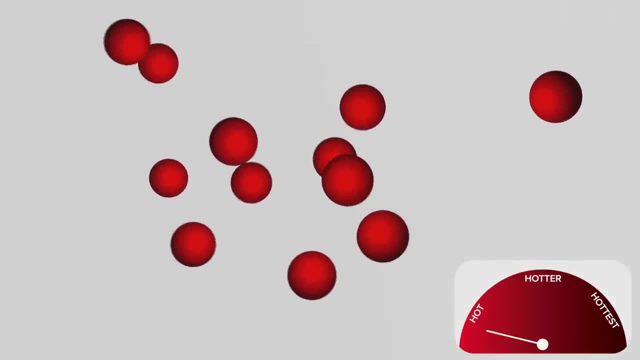 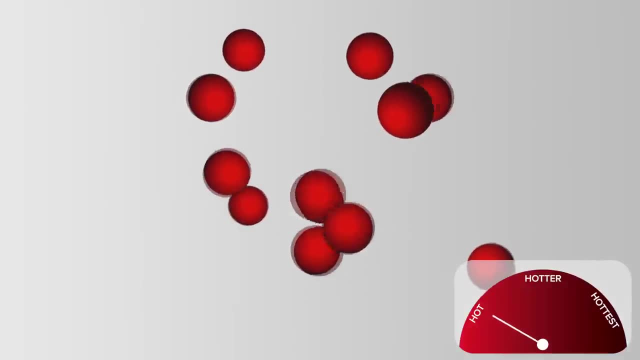 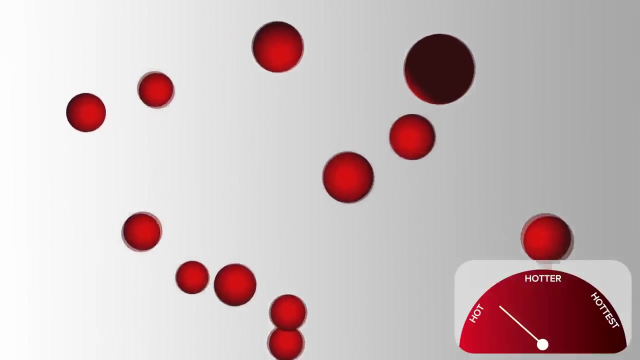 In liquids the molecules have much more energy and the interactions between molecules remain, but dominate less. This leads to phenomenal egg viscosity. When matter is heated even more, the interaction between molecules becomes negligible and matter turns into a gas, with molecules bouncing around randomly. 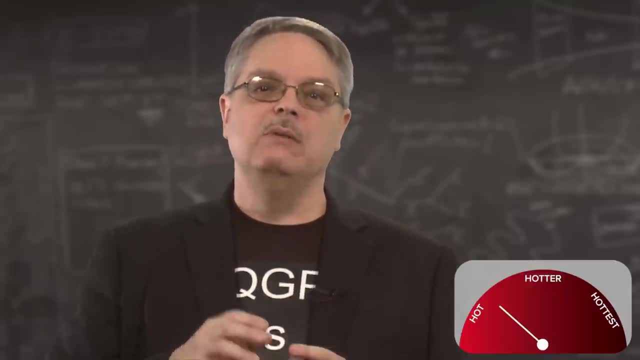 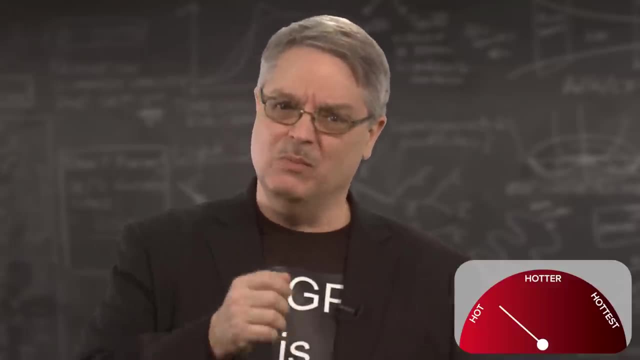 So until now I've described things that you learned about in school, But it turns out that there are states of matter beyond the familiar three. So what happens if we take a gas and turn the heat up even more? To understand this, we can zoom in on a single molecule and see what happens. 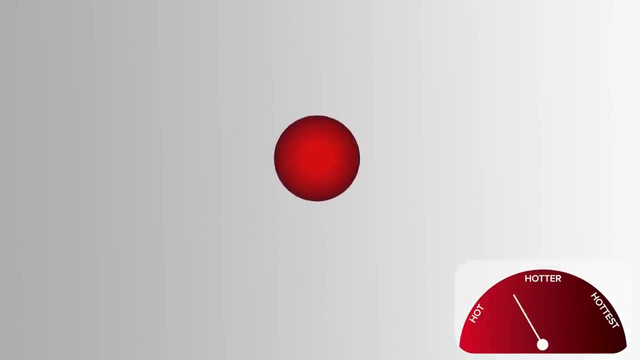 At a certain temperature, the energy is enough to rip molecules apart into their constituent atoms. If one raises the temperature even more, the nucleus of an atom can no longer hold onto the electrons, and the result is that you have electrons running around willy-nilly unbound. 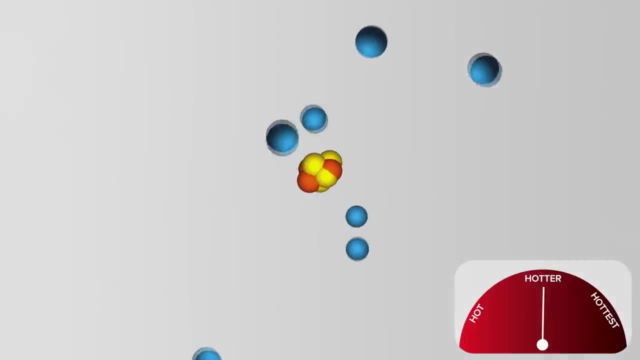 to an atom. The nuclei might initially hold onto some of its electrons, but eventually the temperature will be so high that what you have are electrons and bare atomic nuclei running around. The temperature at which these stages occur depends on the molecules and atoms under consideration. 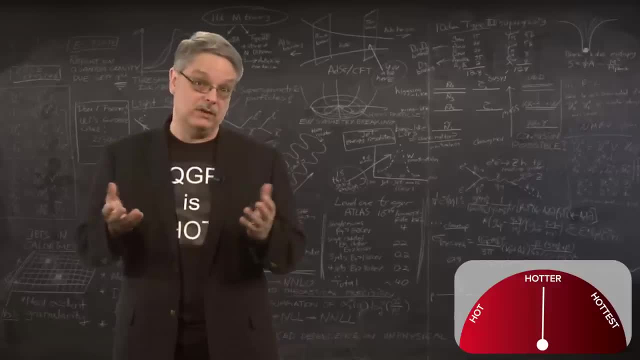 But what I've described here is generally true of all matter. When matter is heated enough that the electrons are being pulled off the atoms, this is a new state of matter called a plasma. You've seen plasma in fluorescent light bulbs, lightning bolts and in those cool plasma. 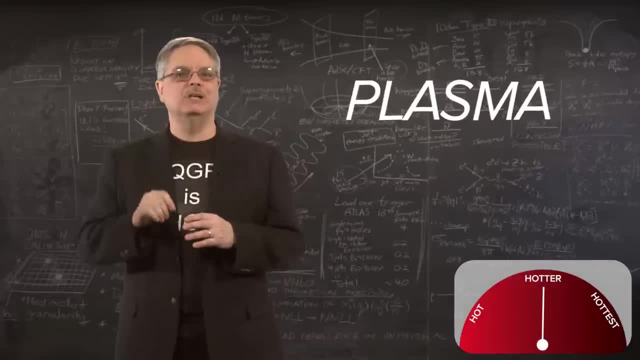 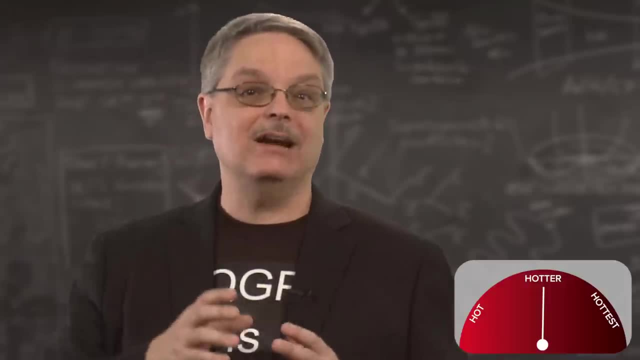 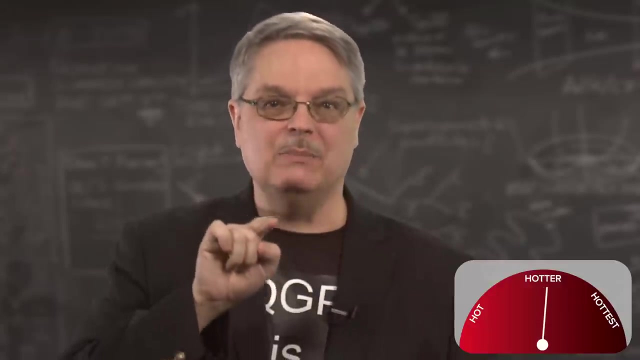 balls. The temperature of the plasma in lightning bolts can be ten times higher than what occurs in a blowtorch. Creating an entirely different new state of matter is pretty amazing. But we're not done. Let's raise the temperature even more To see what happens. then we need to turn our attention to the atomic nucleus. 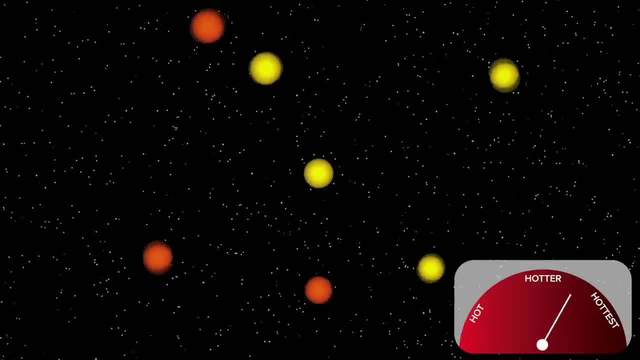 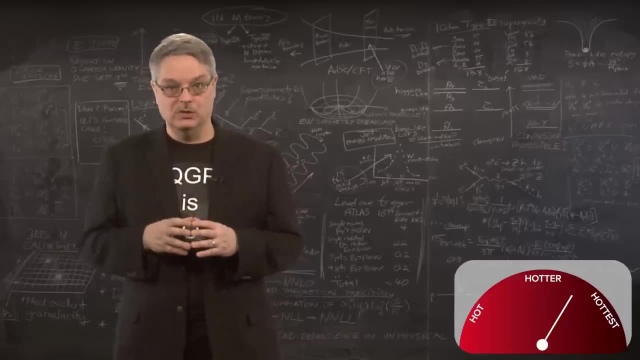 As the temperature increases, the nuclei have so much energy they can no longer reliably hold the protons and neutrons together. But even that amazing achievement isn't the final word. In order to simplify the language, we use the word nucleon to describe both protons. 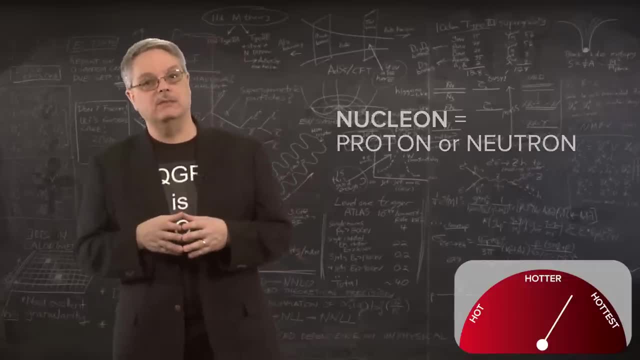 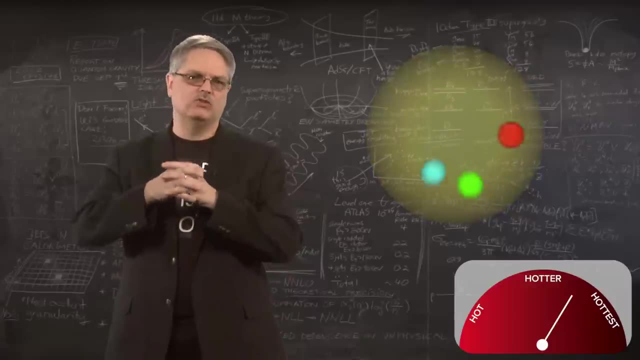 and neutrons. This is because they're both inside the nucleus of an atom. Nucleons are each made of three particles called quarks, and the quarks are held very strongly indeed. In fact, under ordinary conditions one cannot pull a quark out of a nucleon. 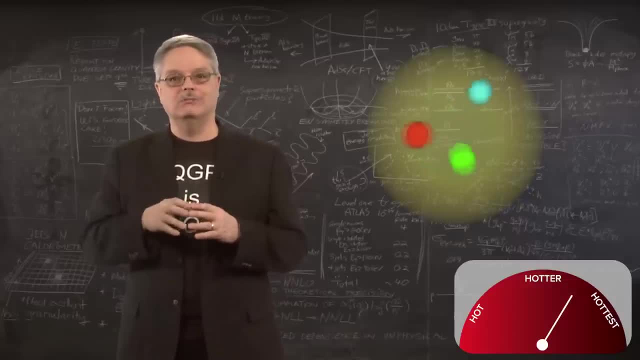 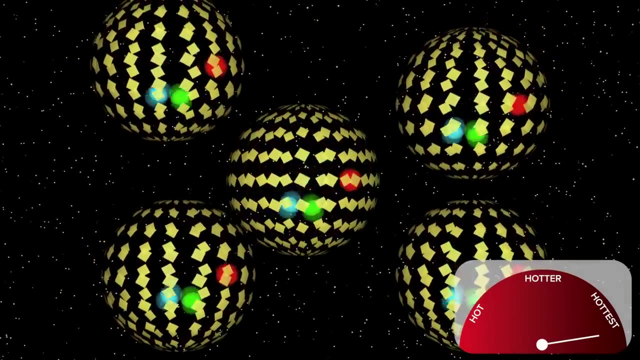 However, the temperatures we can achieve in particle accelerators are anything but ordinary. If we heat matter enough, we can literally melt the nucleons and have the quarks and a particle of force called the gluon run around, no longer bound together. This outrageous state of affairs is a nucleon? 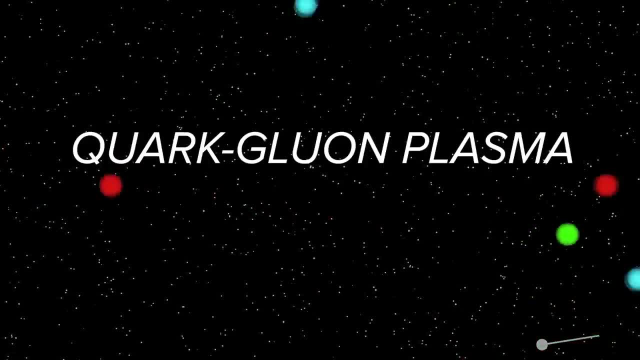 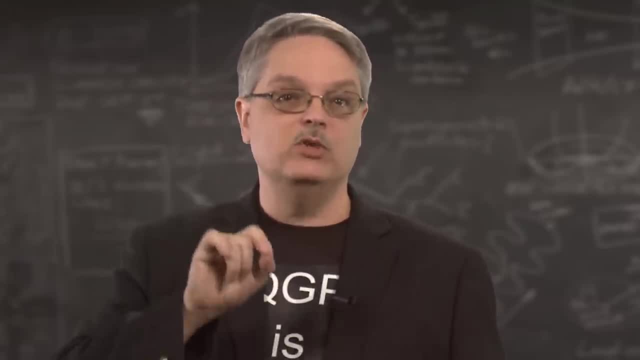 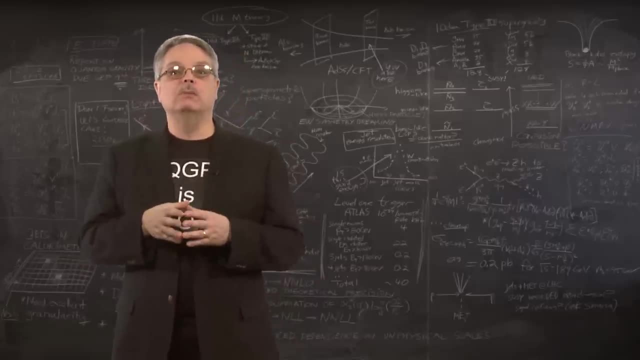 But there is a new form of matter called a quark-gluon plasma. I'll say that again. A quark-gluon plasma occurs when the temperature is so high that individual protons and neutrons literally melt. So you may be wondering if a quark-gluon plasma is a real thing or just an idea. 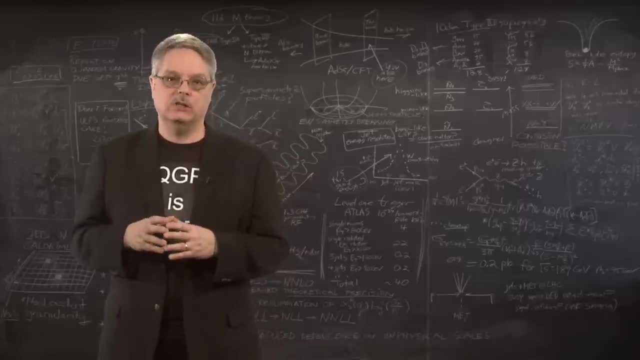 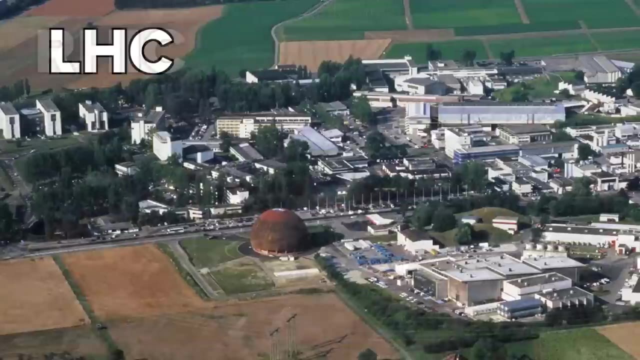 It turns out that scientists can create quark-gluon plasmas that specialize particle accelerators At the Relativistic Heavy Ion Collider on Long Island, also called RIC, and the Large Hadron Collider in Europe, also called the LHC. 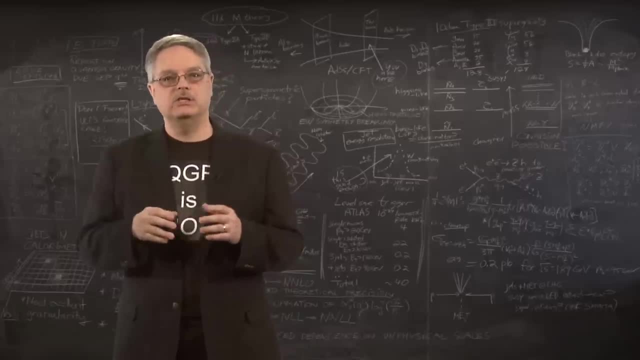 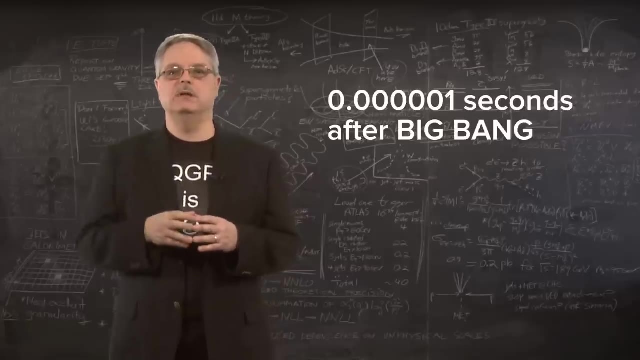 physicists shoot bare atomic nuclei at one another like shooting two bullets together. The temperature in these impacts was last common in the Universe, a millionth of a second after the Big Bang. We see here a simulation of the collision at the LHC, in which two nuclei of lead are. 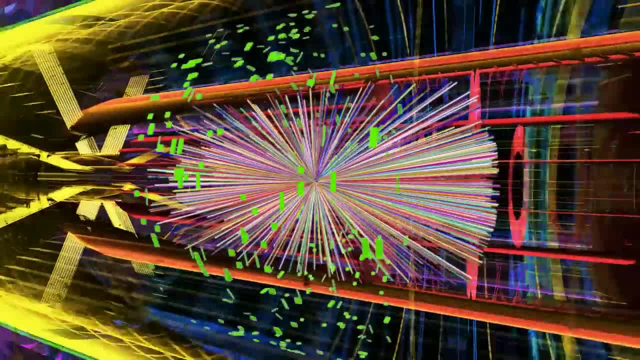 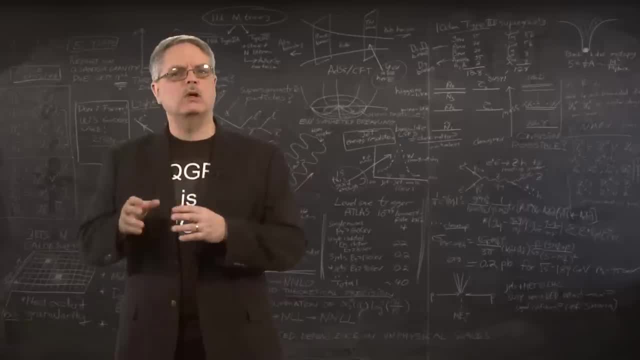 slammed together and a quark-gluon plasma is formed. Physicists generate collisions like these about one month each year. The study of quark-gluon plasma is still a relatively new science, but scientists at RIC and the LHC are studying their data. 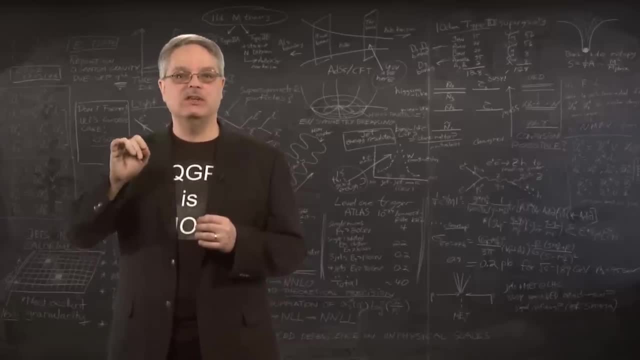 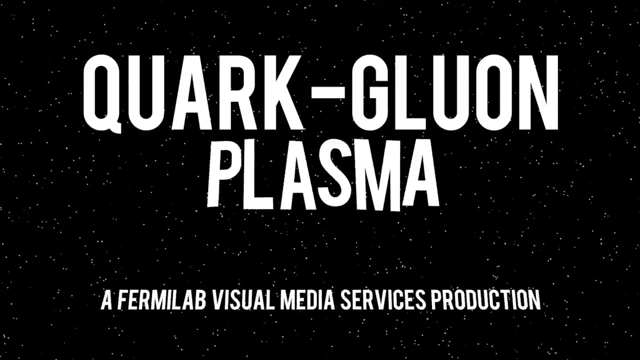 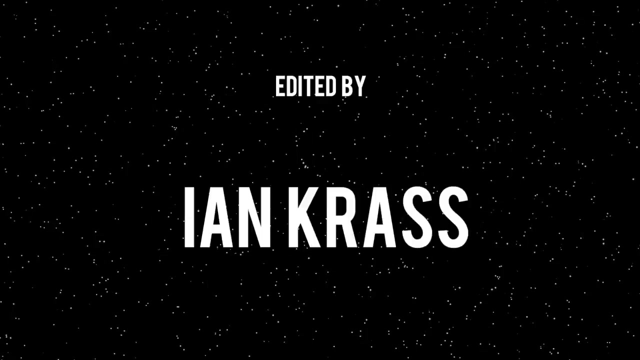 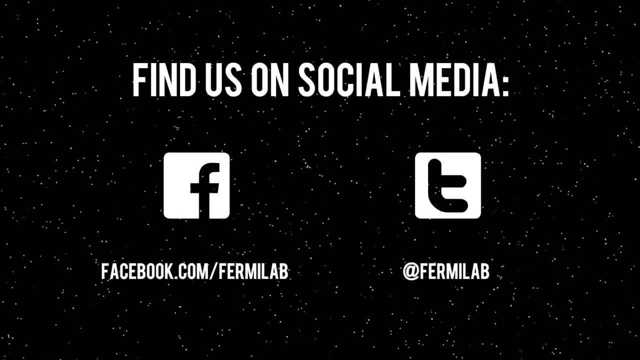 and it is guaranteed that the next few years will teach us something very interesting about this hottest state of matter. And that is totally cool. Subtitles by the Amaraorg community. 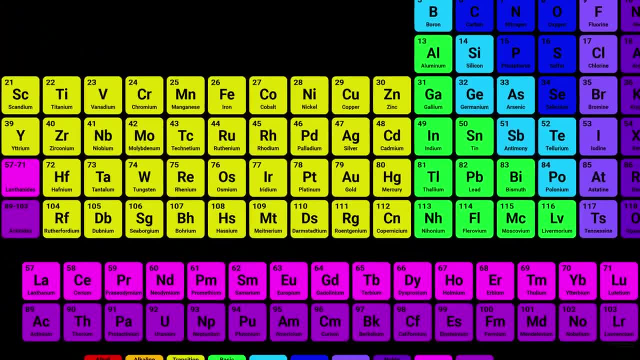 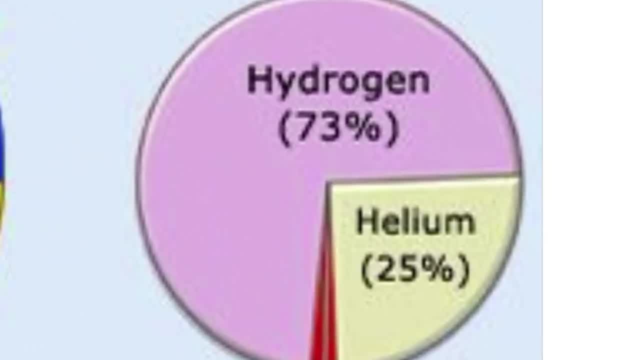 Woo Education. Oh sorry, I get a bit excited when I'm learning, And te- I mean teaching. Yeah, I'm teaching you guys stuff. Alright, guys, let's go. Hydrogen: He's the lightest and most abundant element on the periodic table. 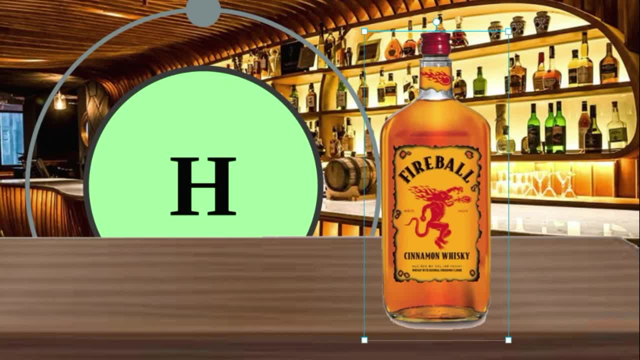 This guy is very chill. He's the life of the party. But you know what? You give this guy a fireball, he's burning. He's full on having a meltdown- Helium. Helium is like the little brother of hydrogen that doesn't have anger issues. 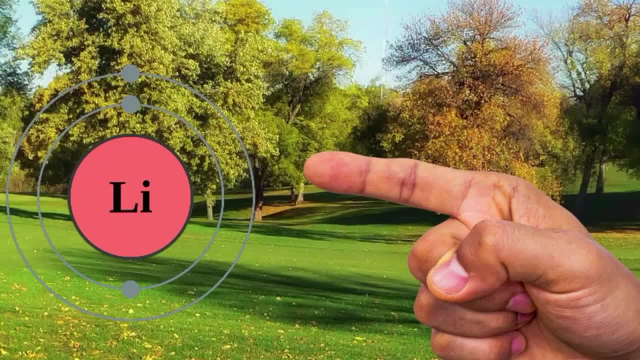 Also he's slightly autistic- Lithium, Very soft metal. but try to be careful when you're around him because if you hurt his feelings or splash water on him he'll probably start sizzling a bit and go cry in a corner. 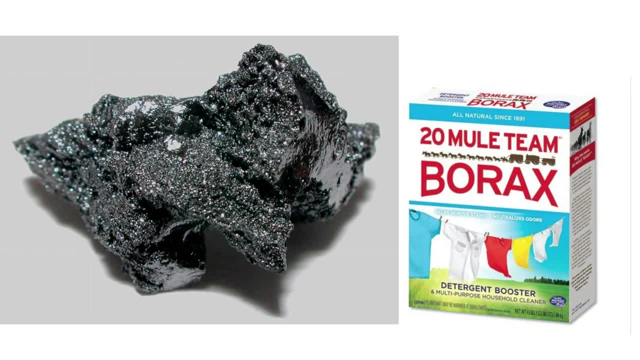 Beryllium, Berylliosis, Boron- Boron is good to clean clothes. Carbon Thanks for existing as the building block of life, so I had to pay taxes. Selfish pr-. Next on the list, we got nitrogen.